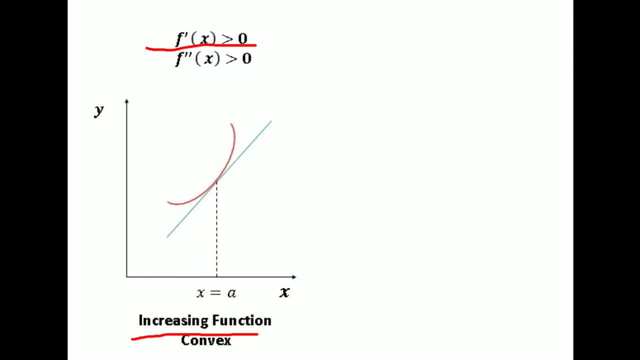 is greater than 0, that is, f prime of x is greater than 0. of course this function is increasing function and a positive second derivative: at x is equal to a denotes the function is convex. at x is equal to a. So this is the increasing function and at the same time it is convex, See the second. 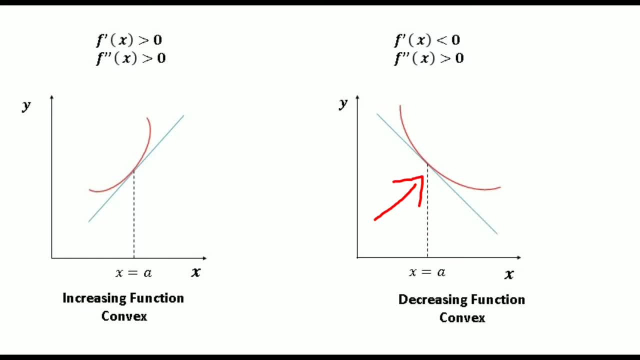 graph, that is the graph of a function which is also lies completely above its tangent line. but the first derivative of a function, f of x, that is f prime of x is less than 0, so the function is decreasing. but we have a positive second derivative at: x is equal to a, denotes the function again it. 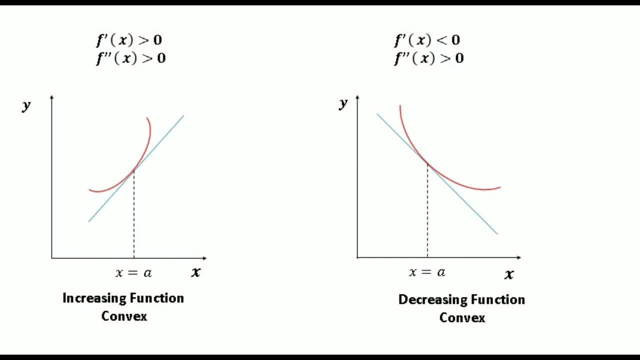 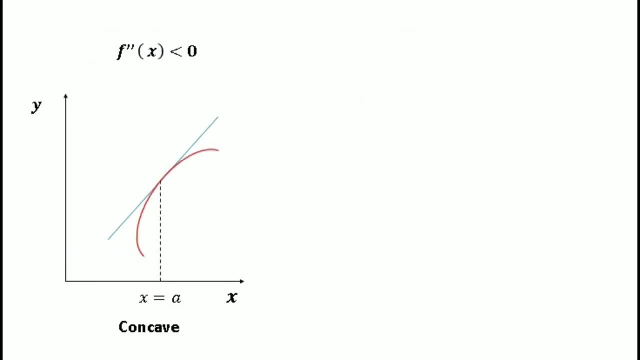 is a convex to the origin at x is equal to a, Although it is a decreasing function, but the function is convex to the origin. A function f of x is concave, at x is equal to a if in some small region close to point a, that is, the graph of the function lies completely below its tangent. 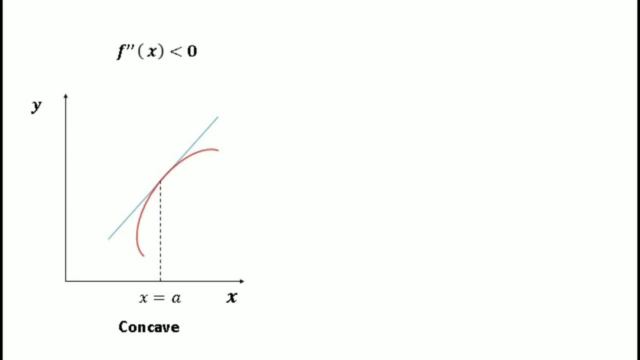 line as against the convex function. So in this case the second derivative, the negative second derivative, at x is equal to a. that is f double prime of x is less than 0, which denotes the function is concave. at x is equal to a. The sign of the first derivative is: 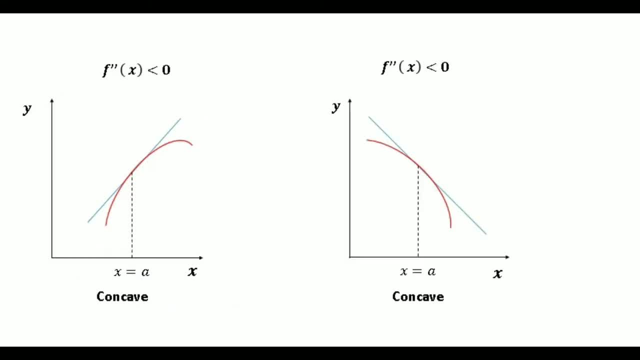 less than 0.. So the second derivative is less than 0.. So the second derivative is less than 0.. Similarly, see the second graph. in this case also, the graph of the function lies completely below its tangent line. So we can say that this function is also concavity, because the negative second 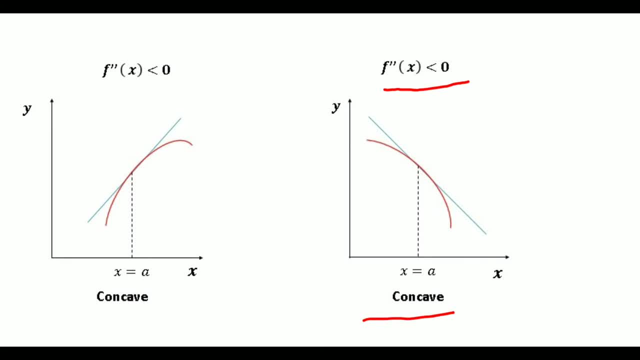 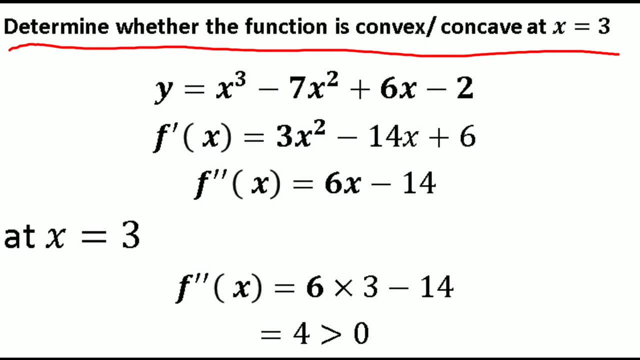 derivative at x is equal to a, that is f double prime of x is less than 0, then, which denotes that the function is concave at x is equal to a, For example. that is, determine whether the function is convex or concave at x is equal. 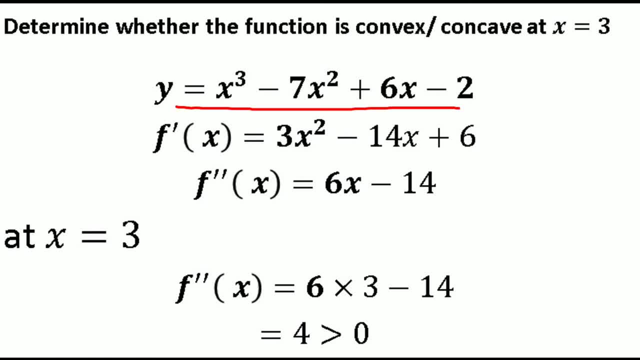 to 3.. For example, the function y is equal to x cube minus 7 x square, plus 6 x minus 2.. So take the first derivative, that is f prime of x is equal to the derivative of x cube, that is 3 x square minus the derivative of 7 x square, which is 14 x plus the derivative. 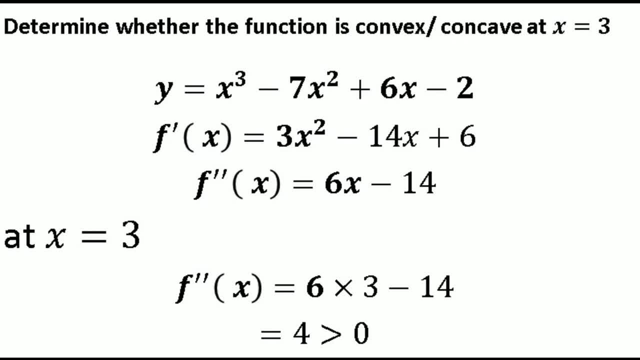 of 6 x, which is equal to 6.. And the derivative of 2, which is equal to 0.. So the first derivative of given function, that is, f, prime of x, is equal to 3 x square minus 14 x plus 6.. Again, we are going to take 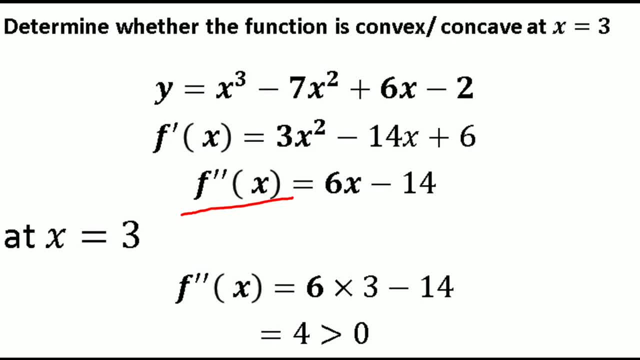 the derivative of the first derivative. So the second derivative, that is f, double prime of x, is equal to the derivative of 3 x square, which is 6, x minus, the derivative of 14, x, which is 14 plus derivative of 6, which is constant, so it will become 0.. 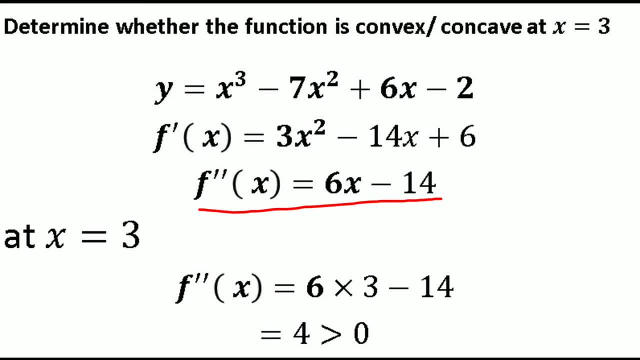 So the second derivative, that is f double prime of x, is equal to 6 x minus 14.. Now we are assuming that x is equal to 3.. Now we are substituting x is equal to 3 on the second derivative, that is f double prime of x. then it will become 6 into x, that is, 6 into 3 minus. 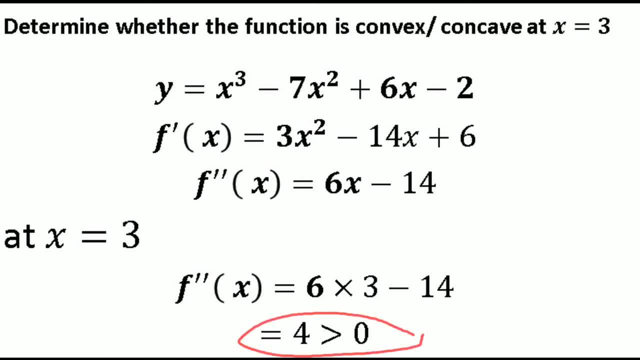 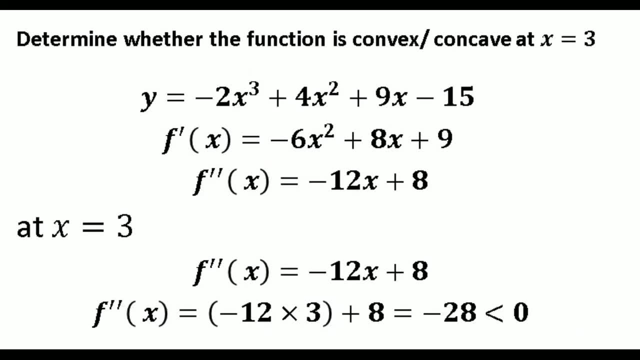 14, which is equal to 4.. Since 4 is equal to greater than 0, the function is said to be a convex function. Consider another example and determine whether the function is convex or concave at x is equal to 3.. So the given function, y, is equal to minus 2 x cube plus 4 x square, plus 9 x minus. 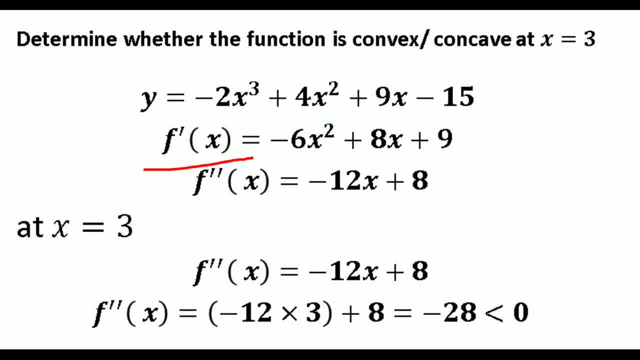 15. Take the first derivative of a given function. then f prime of x is equal to minus 6 x square plus 8 x plus 9.. In order to determine the function is convex or concave, we have to consider the sign of second derivative. 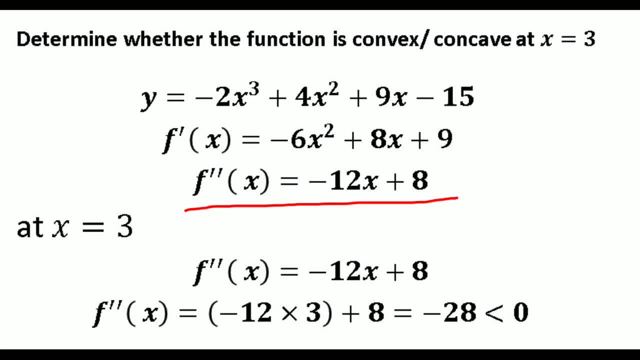 So we are going to take the second derivative. So this f double prime of x is equal to minus 12 x plus 8, and now we are substituting x is equal to 3, then it will become minus 12 into x, which is equal to 3.. So minus 12 into 3 plus 8, which is equal to minus 28.. Since